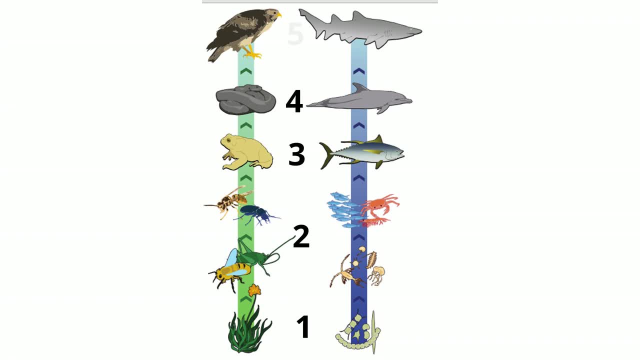 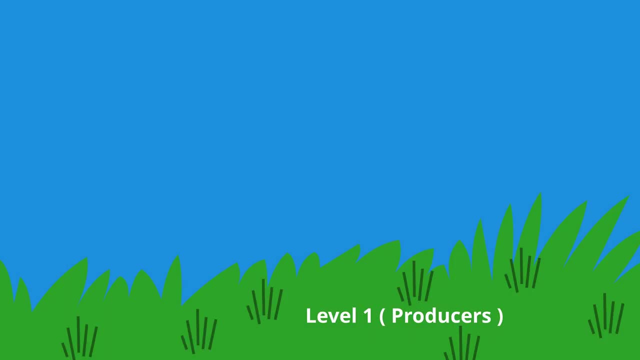 is the number of steps. it is from the food chain's original energy. Let's take a look at these steps that are commonly called levels. Level one: primary producers. Examples include plants and algae that use photosynthesis to make their food. Level two are called primary consumers. 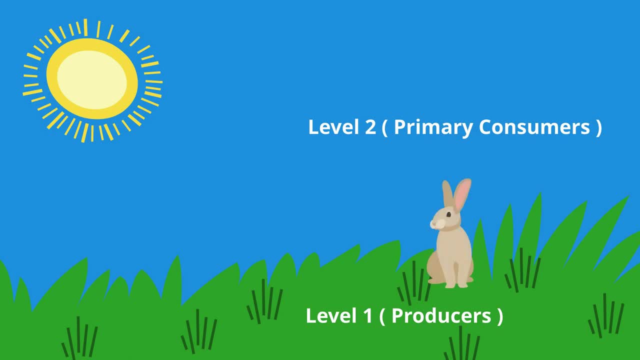 because they eat other producers. These consumers get their energy from eating plants. An example would be rabbits that eat plants. Level three is made up of secondary consumers. They consume level two animals. Carnivores, who are meat eaters, and omnivores are found on level. 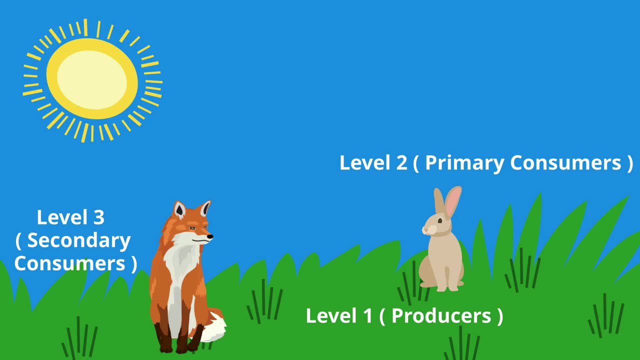 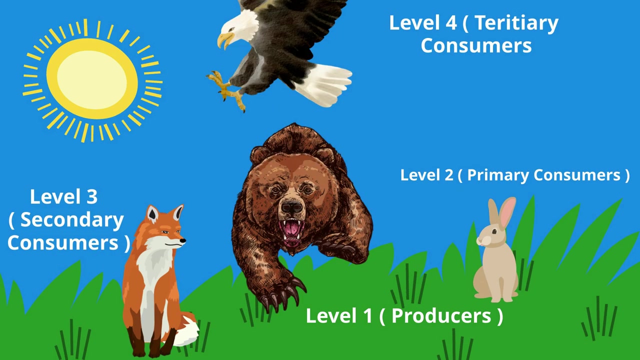 three: Foxes eat rabbits. Level four: this level includes the tertiary consumers. The tertiary consumers eat other carnivores: Golden eagles eat foxes. And finally, level five are called the apex predators and they're at the top of the food chain. They are carnivores without any predators. 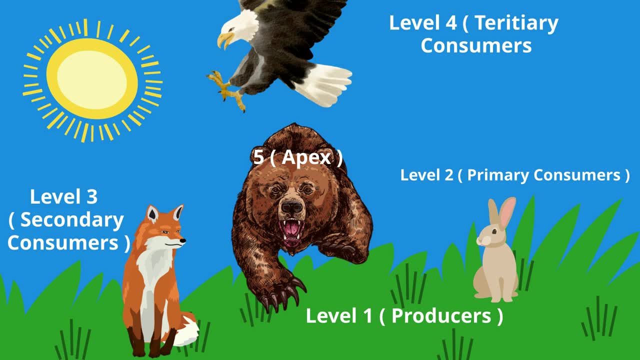 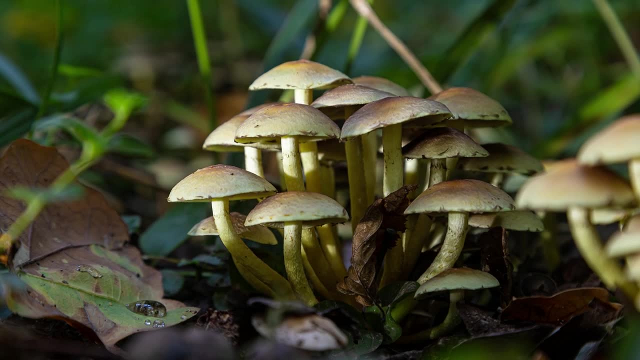 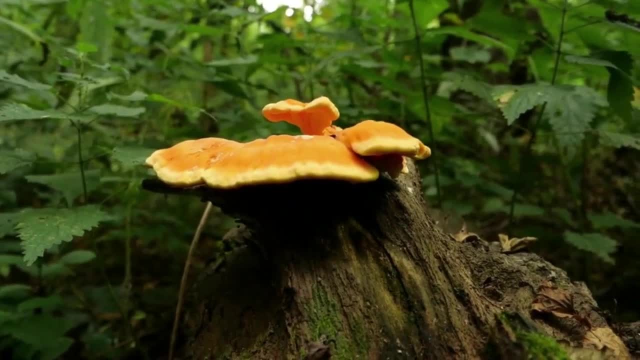 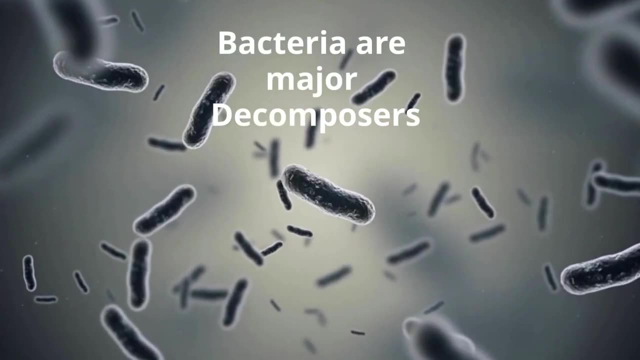 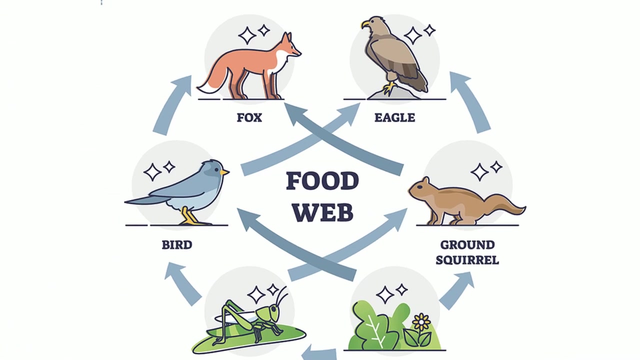 start with primary producers and end with decay and decomposers. Decomposers recycle nutrients that can be reused by primary producers and therefore are essential. A diagram that sets out an intricate network of intersecting and overlapping food chains for an ecosystem is called a food web. 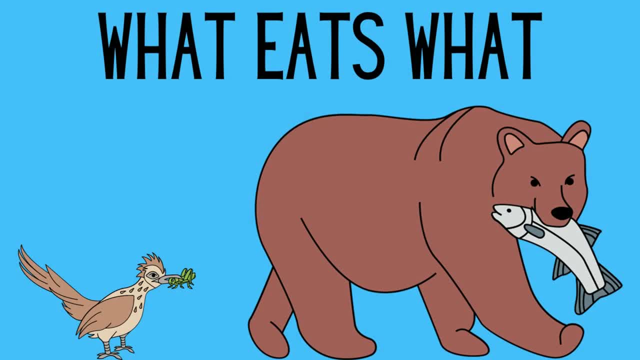 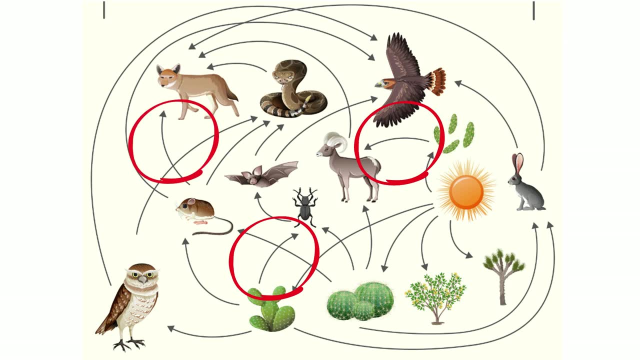 It's basically a visual picture of what eats what in an ecosystem. Let's take a look at a food web. The arrows always point in the direction that the energy is being transferred. You have level one producers that include your plants, and they get energy from the sun.